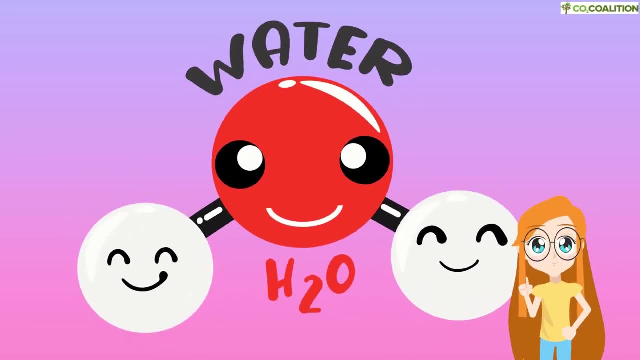 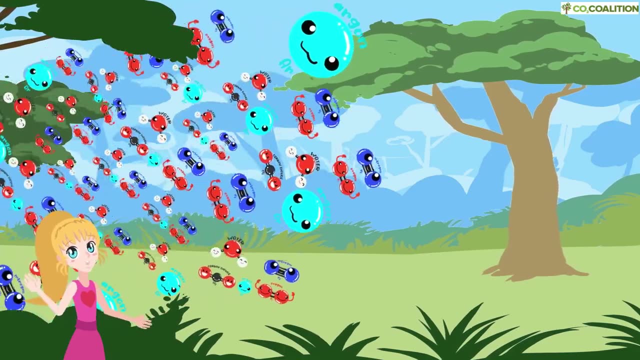 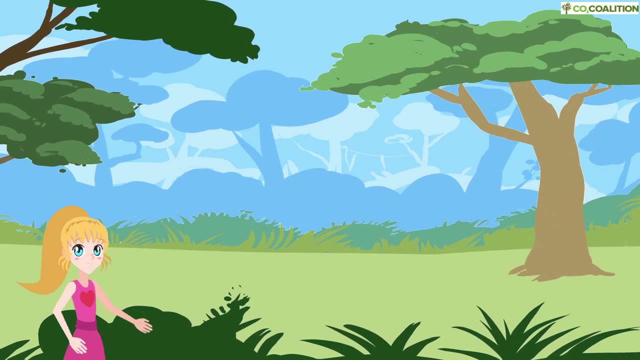 place to place. it is also important for life. Water vapor is invisible, like the other gases. All plants need air to grow. They rely on nitrogen, carbon dioxide and water vapor. They get nitrogen from the soil through their roots. Plants get carbon dioxide through leaves. 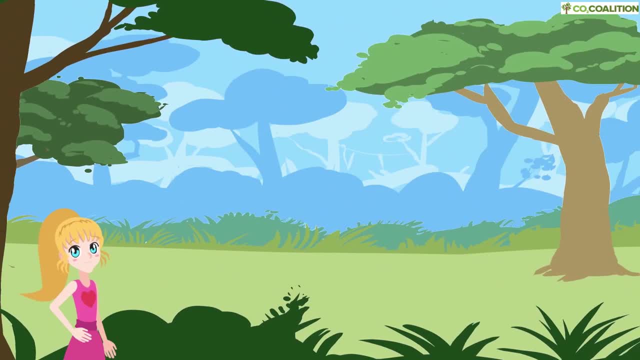 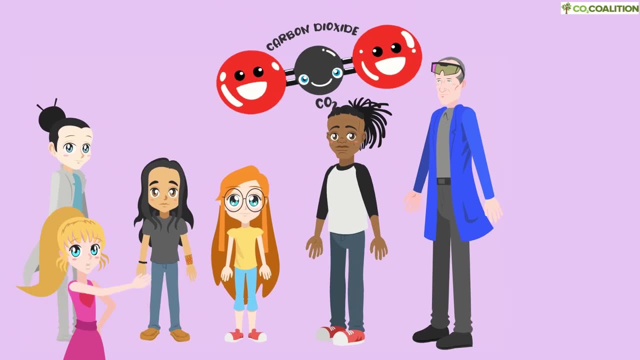 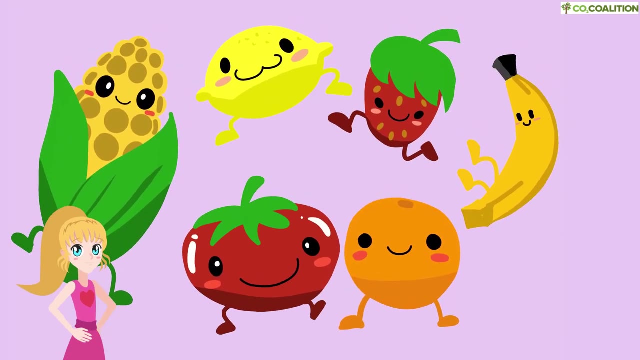 With the help of H2O, it provides food to make them grow. It is the food for grasses that cover hills and prairies, providing pasture for grazing animals. Carbon dioxide supports people. All our fruits and vegetables need it. Without enough of it, nothing would grow. 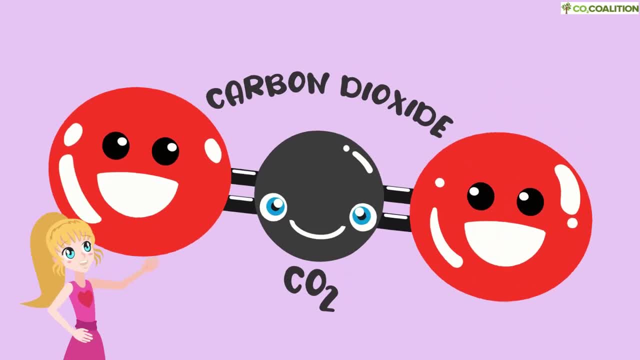 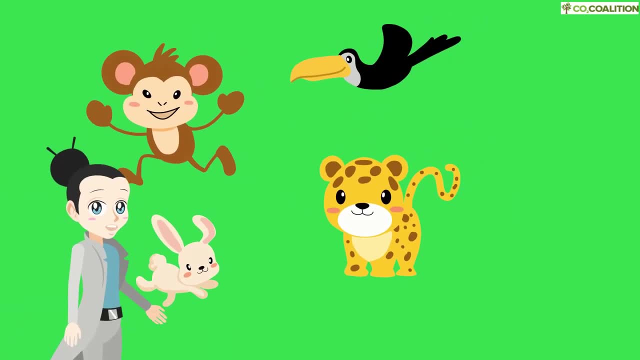 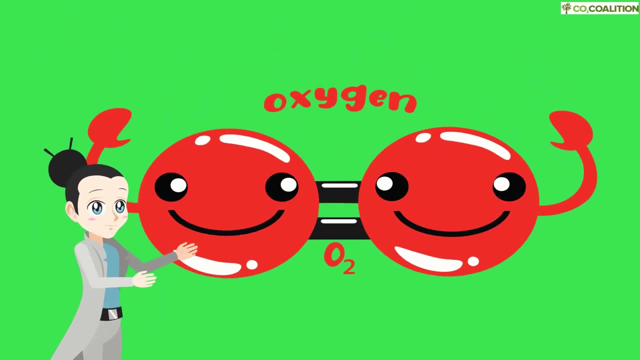 Carbon dioxide is made up of three atoms, one carbon and two oxygen, which, as a pair, we call dioxide. Animals also need air to breathe, but there is just one gas in the air they need. It is oxygen. Wildlife needs oxygen, Birds need oxygen And, of course, 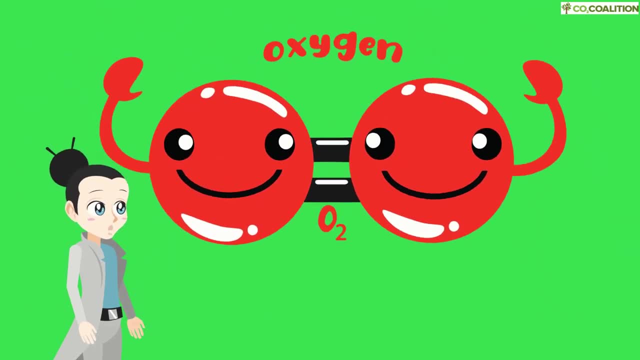 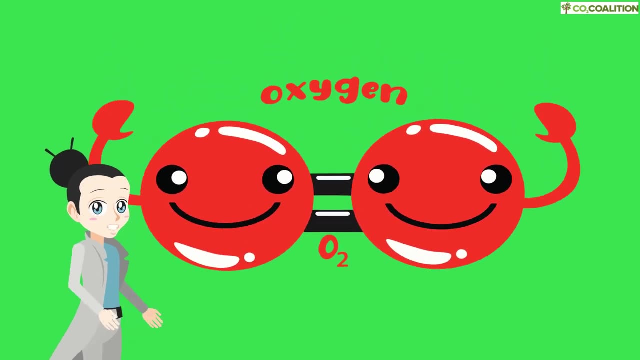 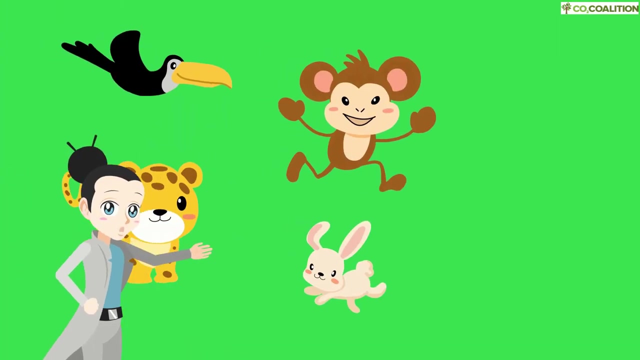 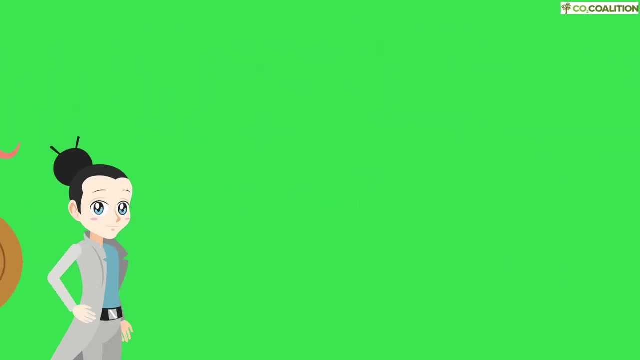 people need oxygen. An oxygen molecule is two oxygen atoms. We could call it dioxide, but instead we simply call it oxygen. Every kind of animal needs oxygen: Every bird, Reptiles like turtles, Wild animals like monkeys, Farm animals, Even the smallest insects like bees and earthworms need it. 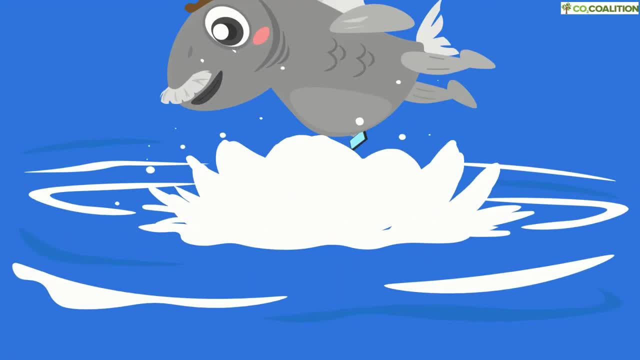 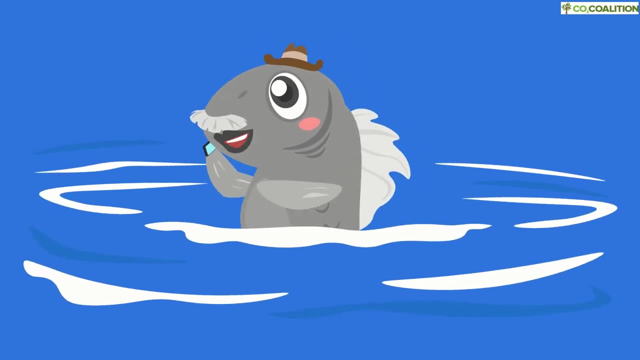 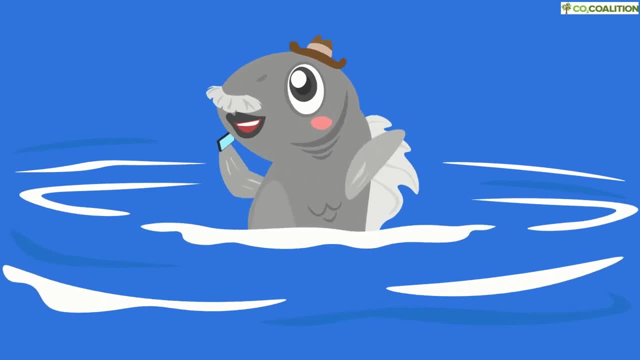 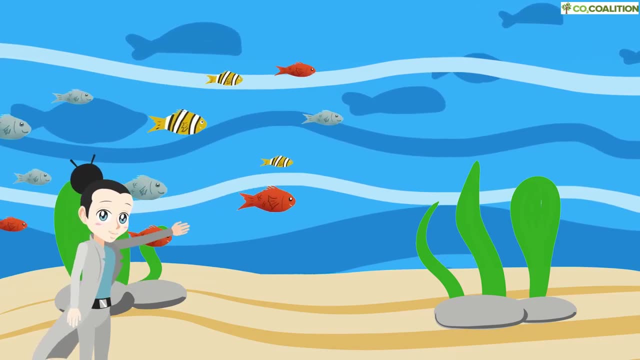 This is not about land animals. It's about sea life. After all, oceans cover most of the planet. Oh thanks, Mr Fish. Of course, Ocean plants like kelp also use carbon dioxide, Like plants on land. sunlight energy converts. 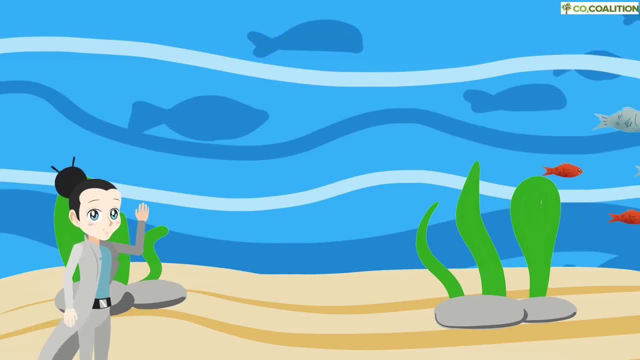 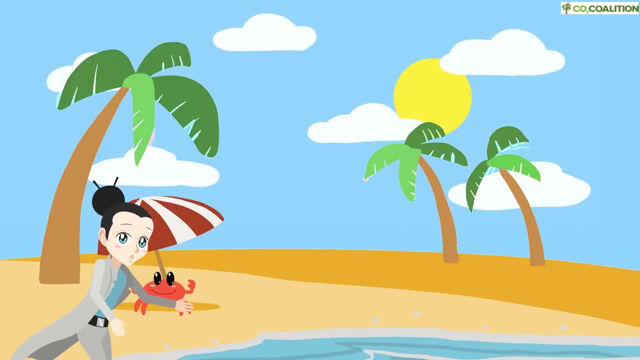 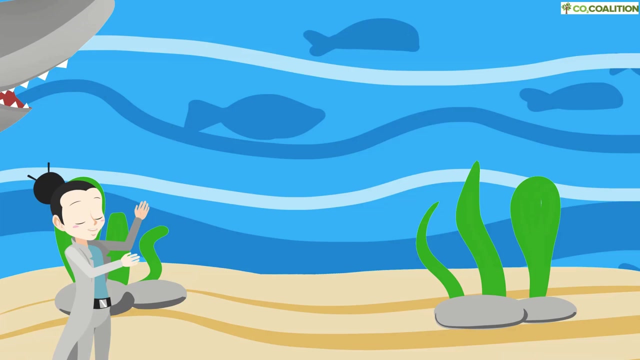 carbon dioxide into plant food, a process known as photosynthesis. Sea creatures must have oxygen. The water in oceans and lakes can absorb carbon dioxide, and oxygen from the air can get oxygen from the water. so do all the fish, from the smallest minnows to